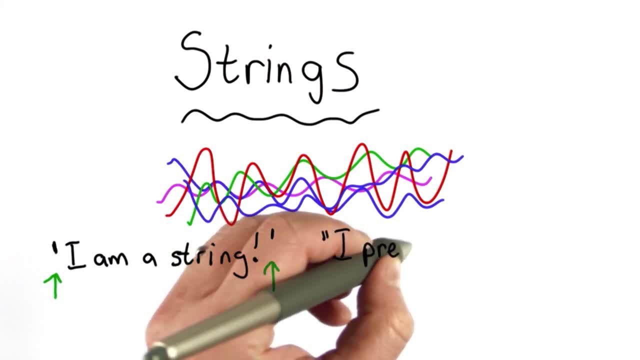 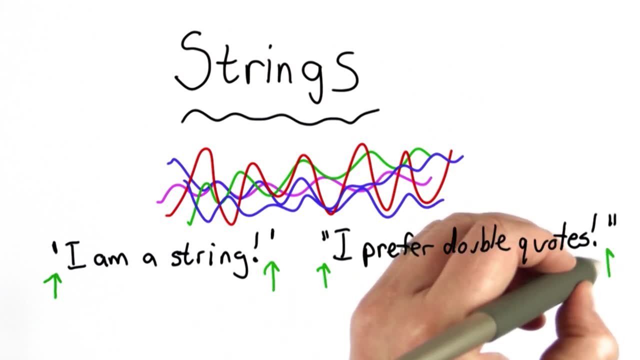 of characters between the single quotes. If we want, we can use double quotes instead. If we use double quotes, then the double quote starts the string. We can have a sequence of characters and a double quote that ends the string. The only requirement is that if we start the string with a single quote, it has 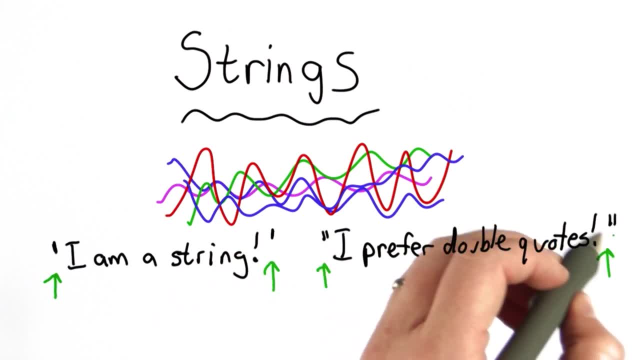 to end with a single quote. If we start the string with a double quote, it has to end with a double quote, And that's actually a handy property because that means we can have the other kind of quote within our string. The string starts with a double quote It. 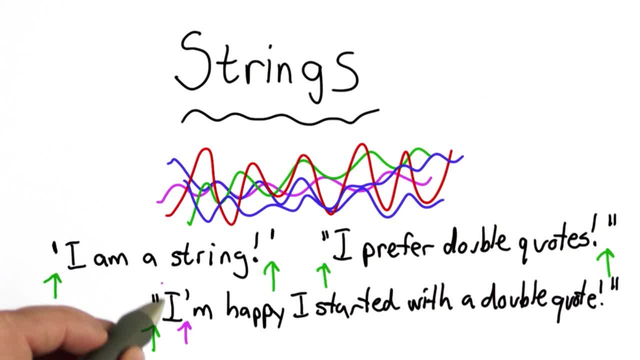 contains a single quote inside it. but because we started with a double quote, that single quote doesn't end the string. That single quote is just like another character in the string. The string continues until the closing double quote. So let's try some things in the Python interpreter So we can print a: 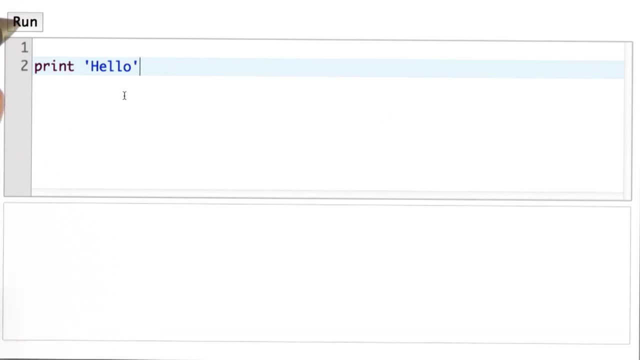 string, just like we can print a number. So here I'm printing the string hello And when we run this we see the output hello. It's printing hello. We don't see the single quotes as it prints, but we know that it's a string that. 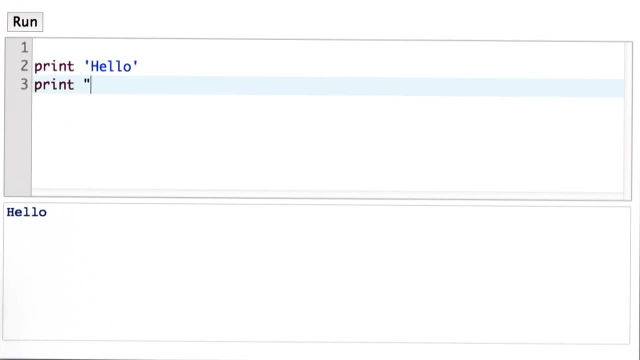 was printed. We can print a string with double quotes. And one thing to notice: when you enter strings in the interpreter, the color is black. now, Since it's an open string, it hasn't been finished. Once I type the final quote, that 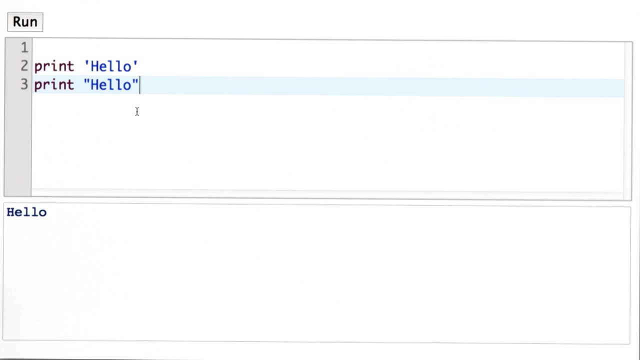 closes the string, the color changes to blue. So now when we run this we have two prints, both that print. hello, It looks the same both times. It doesn't matter if we use single quotes or double quotes around our string, Just. 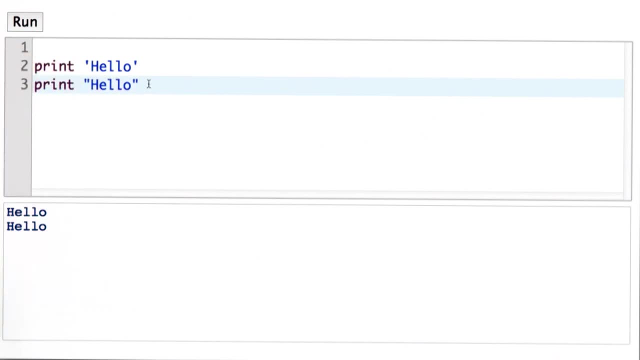 to check everyone's paying attention. I'm going to try one more thing Now. I'm printing hello without the quotes. Try to see if you can guess what that will do. We won't make a quiz of this, but try to guess before I run it. Now that I run, 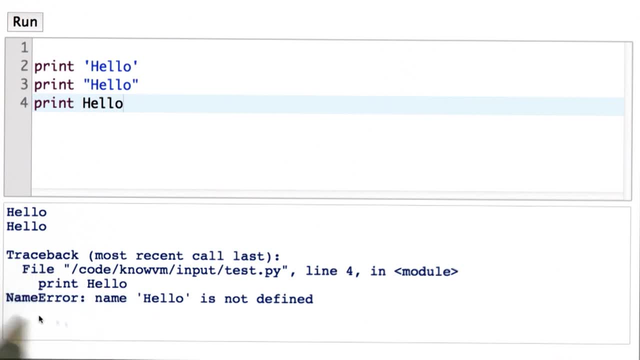 this. we see the result: We get a name error. The name hello is not defined Without the quotes. this looks just like a variable. It's a name, but it's a variable that we didn't define, So when I try to use it, I get an error that the